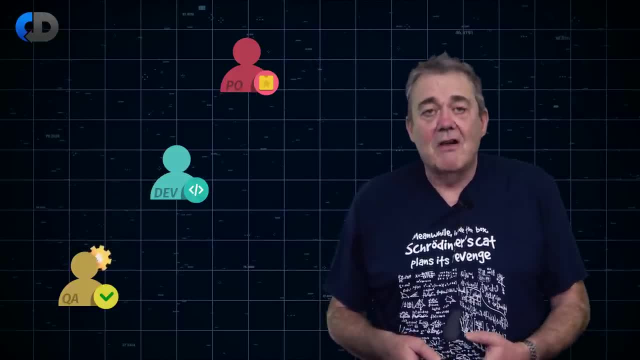 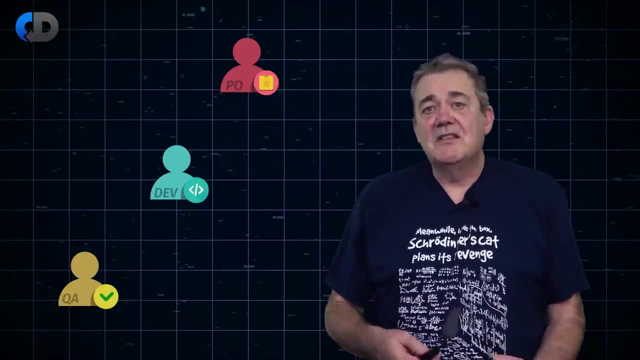 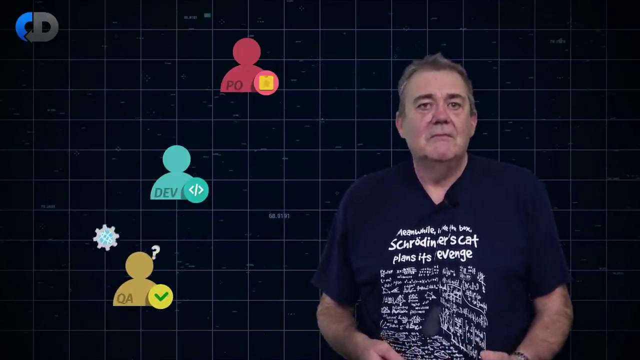 plans. Developers need to shape their work and their software so that release can happen at any time, maybe even in the middle of the development of a feature. Testers and QA people don't act as gatekeepers to release into production. Hang on a minute. isn't that what QA teams do? Well, no, 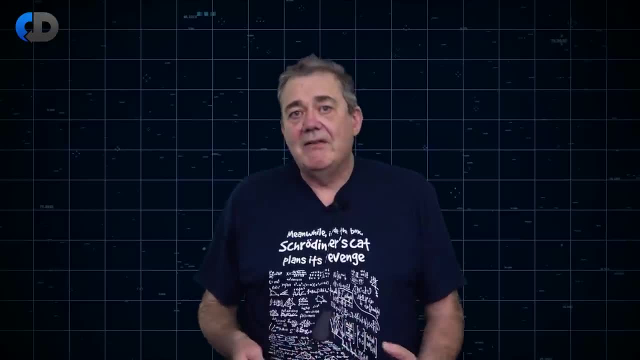 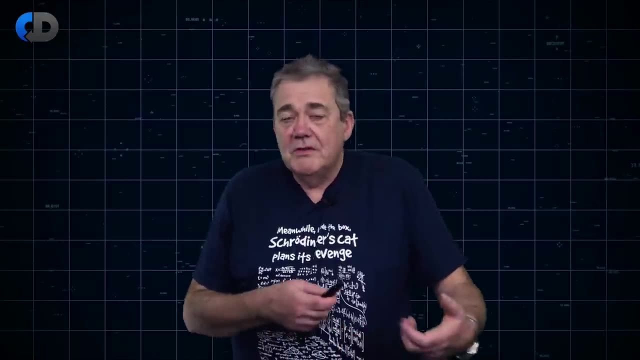 not in continuous delivery teams. Let's think about this from first principles. If our aim is to work so that our software is always in a releasable state, then we need to think about what does releasable really mean? It's clearly contextual. It will depend on the nature of 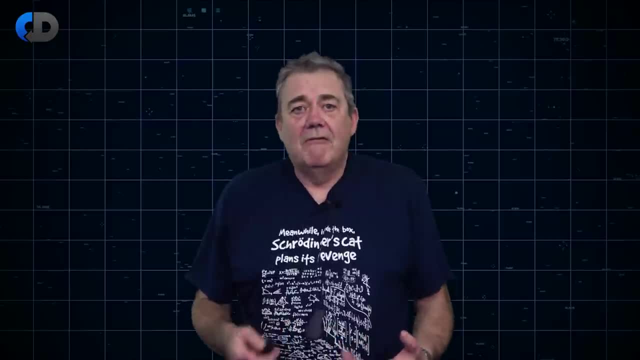 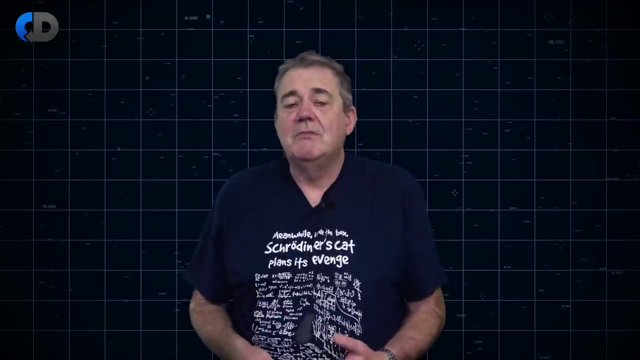 your software and the nature of your organization. But the most obvious definition is if that we think our code is releasable, it means that there's no more work to do before we're happy for it to be released. No more testing, no more documentation, no more sign-offs: It's ready to go. 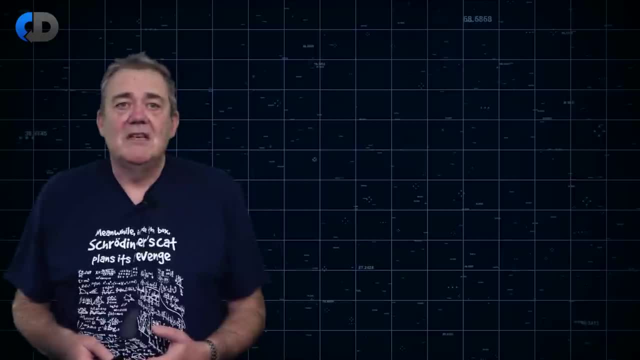 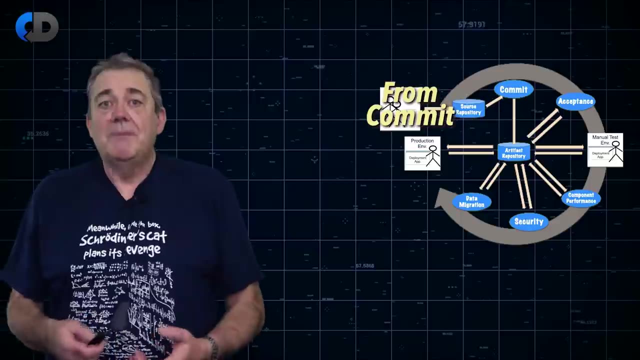 The way that we determine the releasability of our software in continuous delivery is to create a deployment of our software. If we think our code is releasable, then we need to define what releasability means for our software. The deployment pipeline is definitive. It goes. 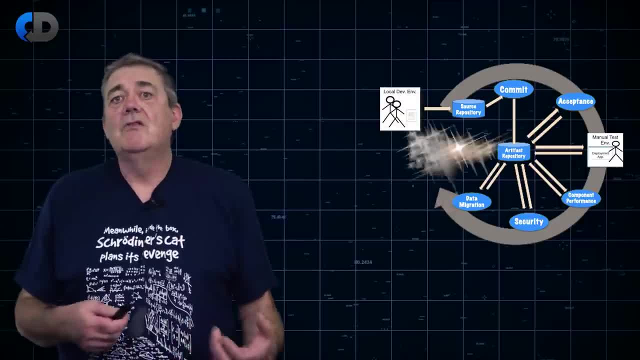 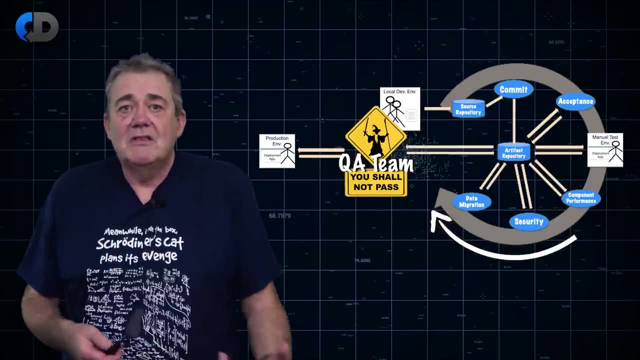 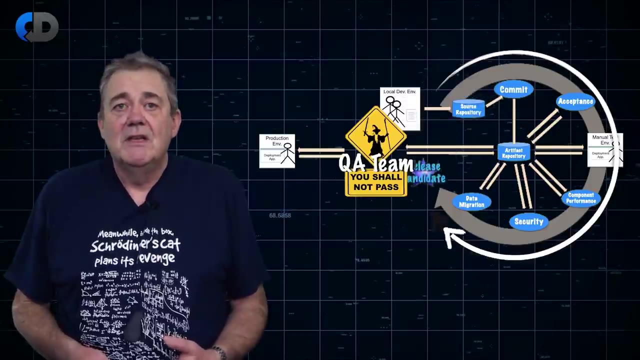 from commit to releasable outcome. It's no good building a deployment pipeline that looks like this, because at the end of the pipeline, QA could still reject the change. Our change is not releasable, and so the deployment pipeline is not definitive. This adds complexity to the development. 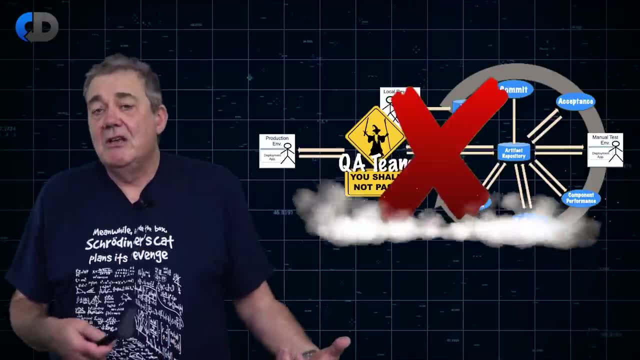 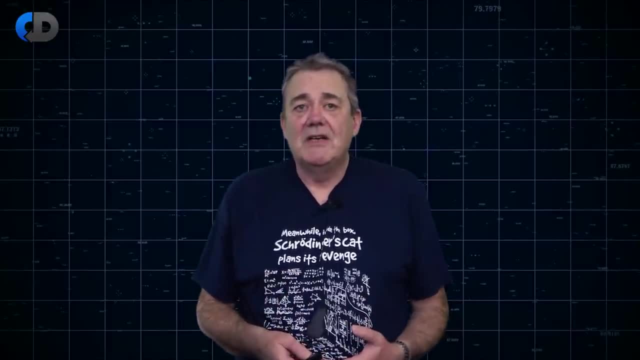 process lengthens the feedback cycle and delivers bad news. If we think our code is releasable, it means that there's no more work to do before we're happy for it to be released. Whatever, it is that it takes to figure out if your software is releasable. it almost certainly involves two kinds of check: Does the software do what we meant it to do, and does it still do what it used to do before this change? For many more traditionally structured teams, finding the answers to both of these questions is often left to a QA department, or at least QA people looking at the software. It's a good idea to think about this first before you start to work on a project. Most teams, even most agile teams, treat QA as some kind of gate into production. The role of QA is to find the answers to these questions After the development on new features or bug fixes is complete. 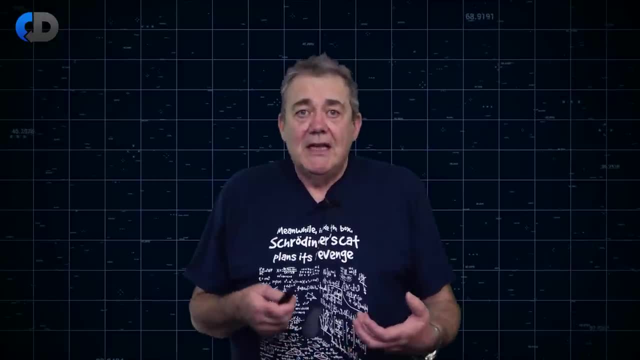 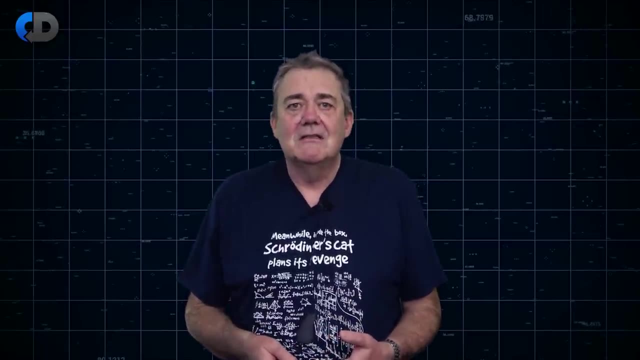 This is problematic. It doesn't really work very well. It seems obvious that we should organise things this way, but when you stop and think about it it doesn't really make much sense. Let's imagine then that we're building a software that's not really a regular 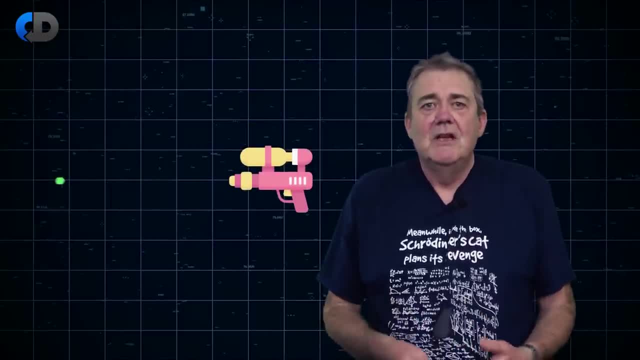 a regular-level software. It's a very complex, complex, complex, complex structure. It's a very complex that we've been tasked with creating some green dots. We begin churning them out, but at some point during the production run. 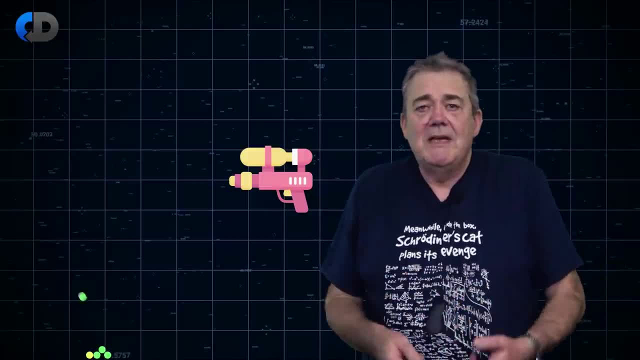 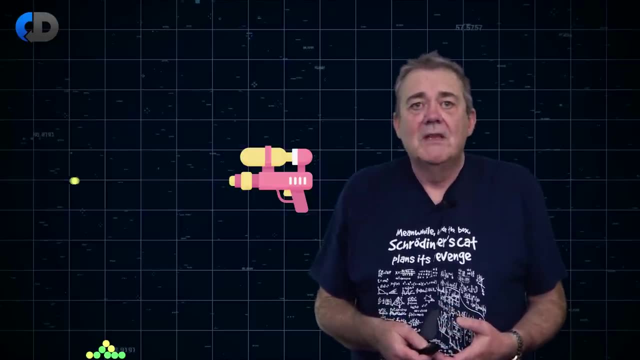 we run out of blue dye, So we end up with some of our dots being yellow by mistake. The longer we wait, the more yellow dots we make, until they're all yellow. So the bugs in our system, the yellow dots, grow until they overwhelm the system. 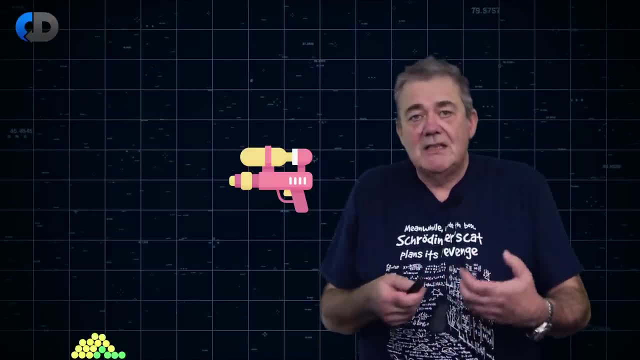 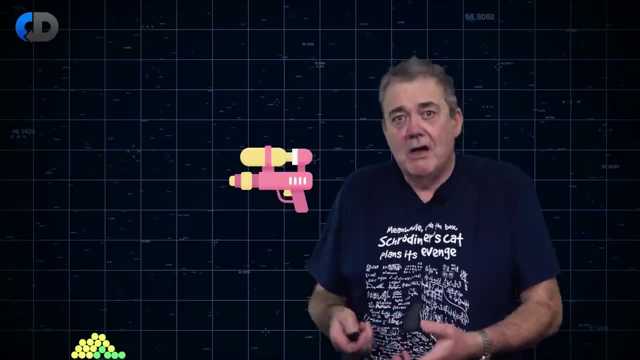 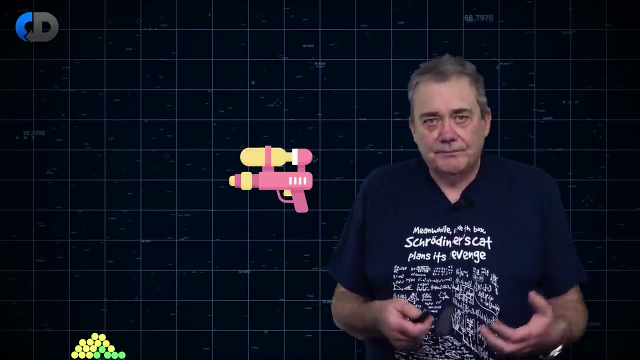 How could we prevent this? Well, obviously this is a time-sensitive thing. The longer we leave things before we notice the problem, the more waste yellow dots we will have created. So if it takes one week for the blue paint to completely run out, 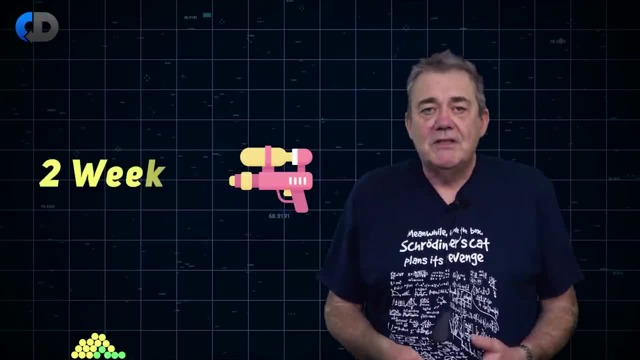 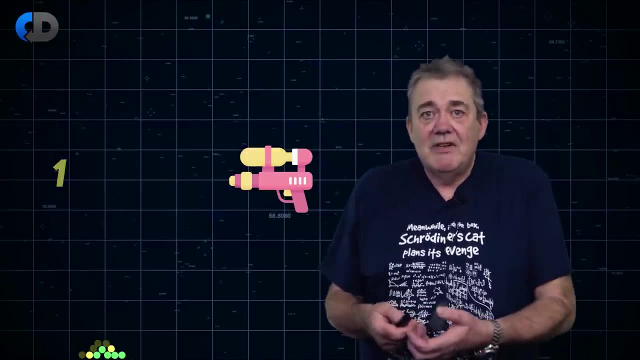 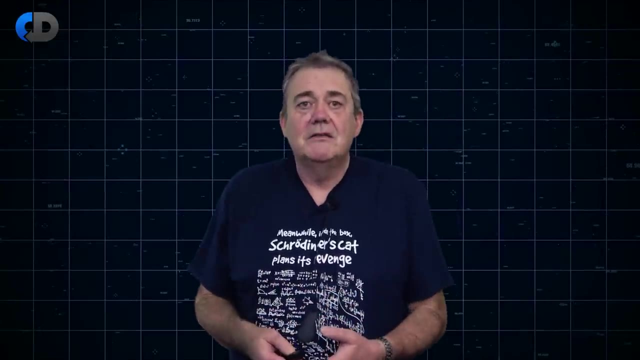 but we only test every two weeks. nearly all of our output is gonna be waste If we test every week. a big fraction of our output is waste If we test every day, maybe only a few dots were waste. So the frequency with which we test matters a lot. 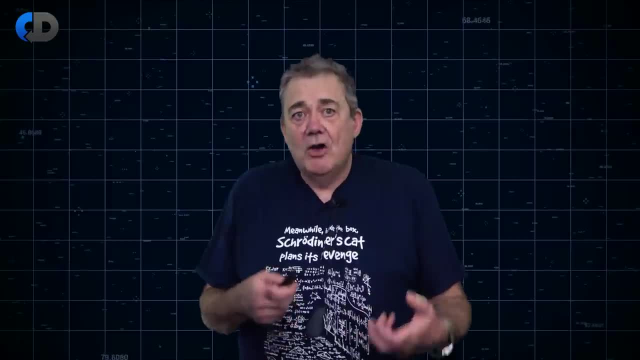 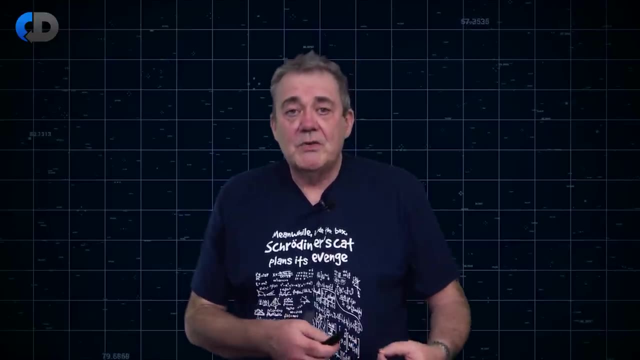 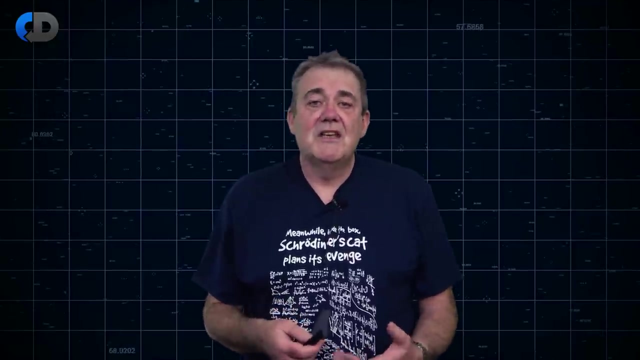 If we want to make high quality products, we need to up the frequency with which we test them. A better way to think of this is that we want to reduce the time between making a change and testing that the change was correct. So what if, instead of testing our dots every day, 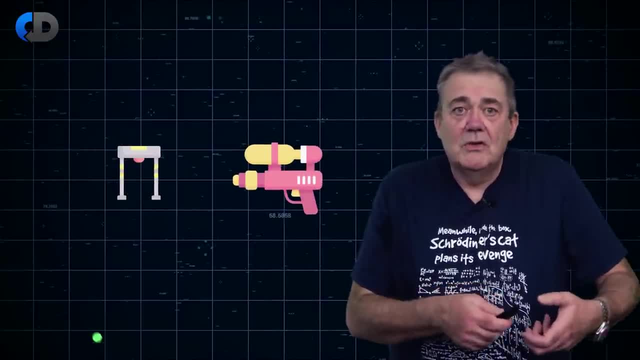 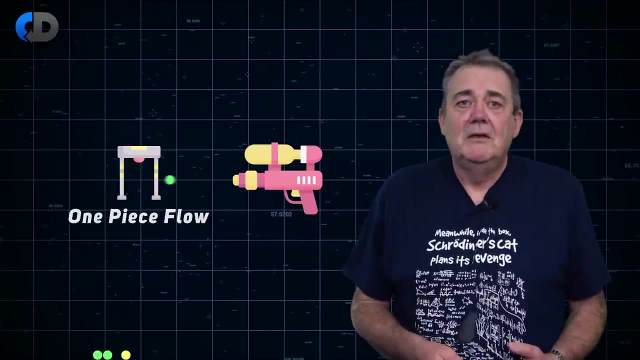 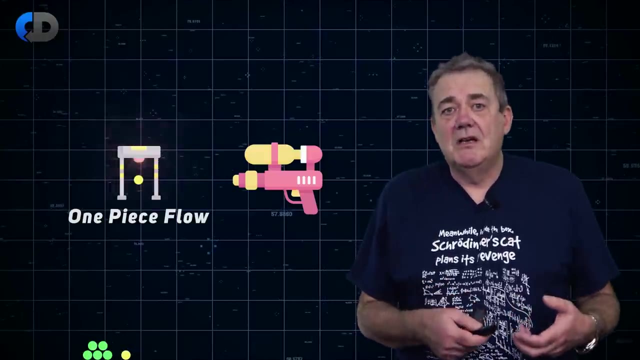 we tested them as they were being produced. As soon as we saw a problem, we stopped and fixed it. This is what lean people call one-piece flow. Instead of testing changes in batches, we're gonna test every change Now if a problem occurs, like we ran out of blue dye. 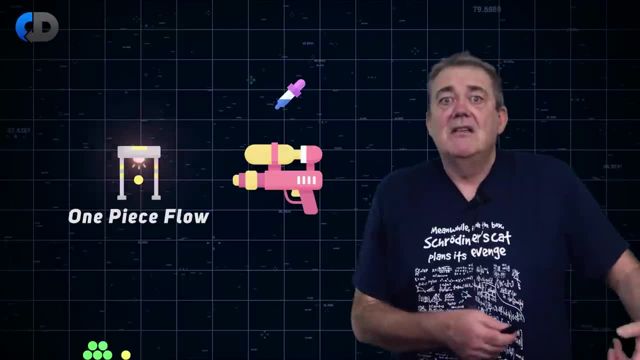 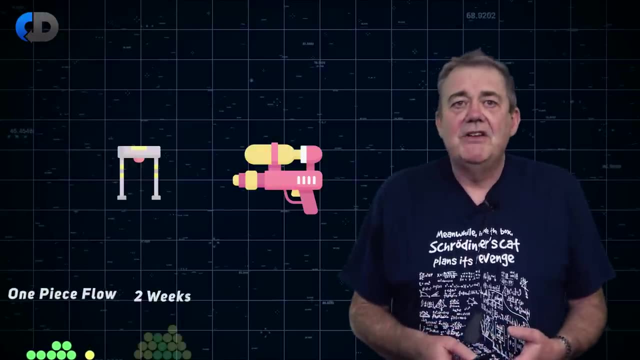 we're gonna stop, add blue dye and then continue having had a single failure. When you think of it like this, it's obvious that check every change will result in higher quality. Our aim, then, is to identify a mistake at the early stage. 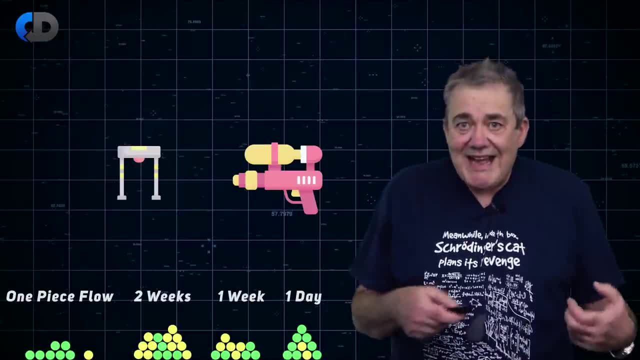 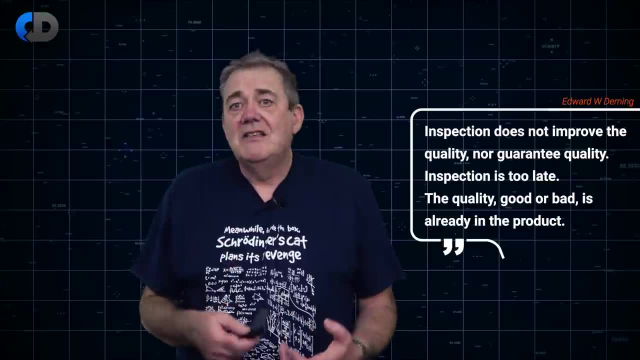 That's the earliest possible opportunity. The earliest opportunity is at the point when we make the change. To put that in another way, as Edward Deming said, you can't inspect quality into a system, you build it into the system. This is true. 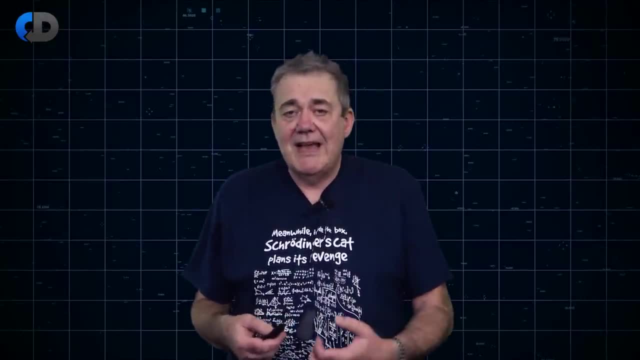 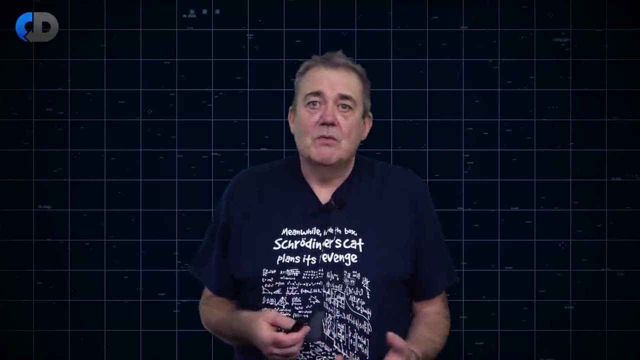 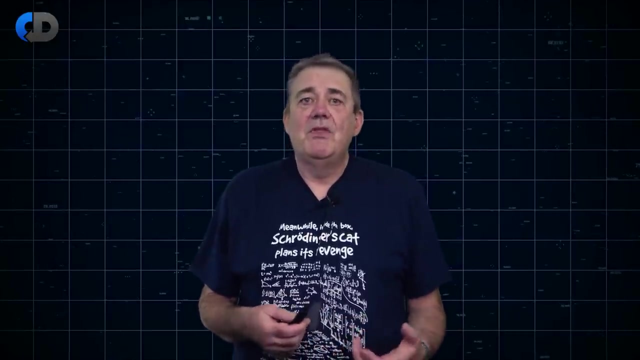 However good your QA team or tests, they will spot mistakes after they happen. What if, instead, we could spot mistakes while we were making them? That's what Deming really meant. We build error detection into the process of creation- The people that make these mistakes. 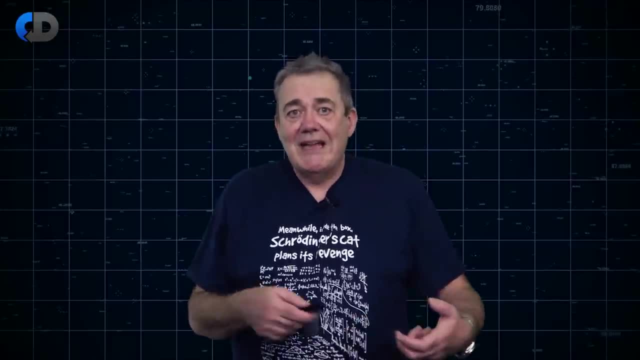 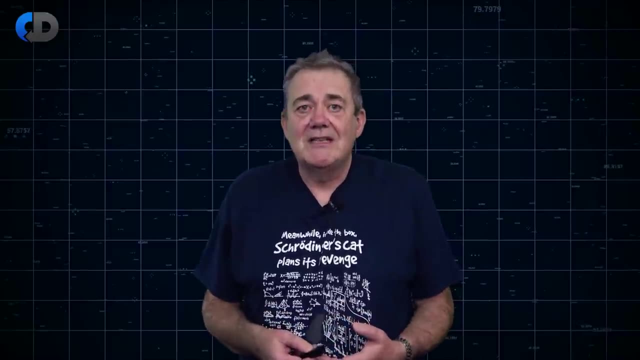 are the programmers that put them into the code, So we need to catch them then as the programmer introduces them, So we can do things like pair programming and automated testing to catch the mistakes as we are making them. How far can we take that? 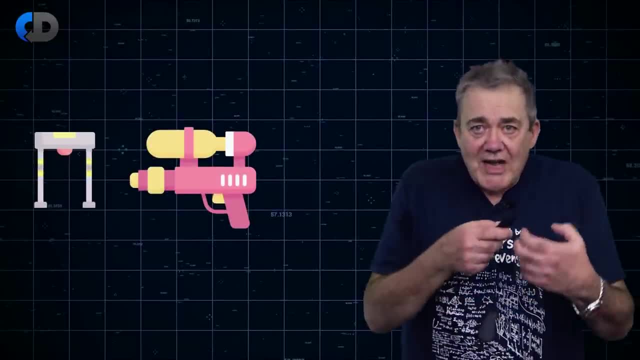 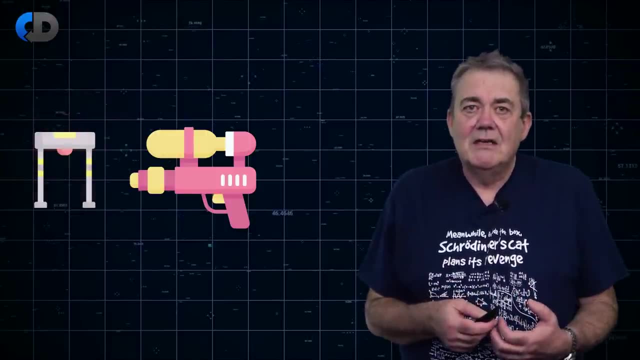 Well, let's go back to our green dots for a minute. We could check each green dot after it was finished to see if it matched our standards. But could we do any better than that, Assuming the green dot took time to create? 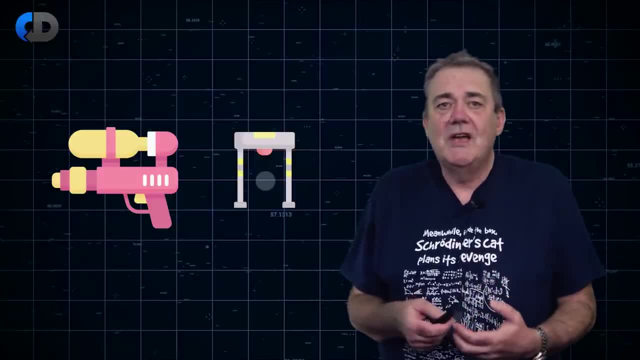 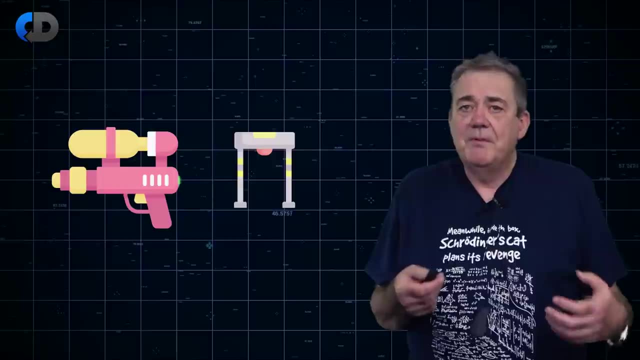 then we could monitor the quality of the dot during the course of its creation, And as soon as we saw something that we didn't like, we could correct it. That's the step that test-driven development takes. Not only do we test every change, 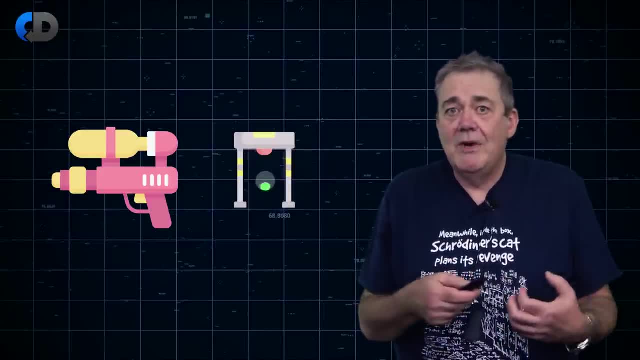 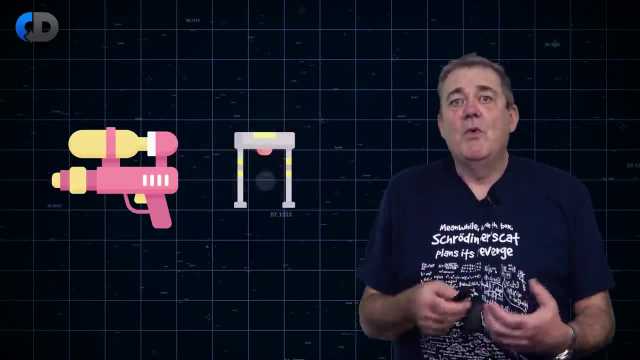 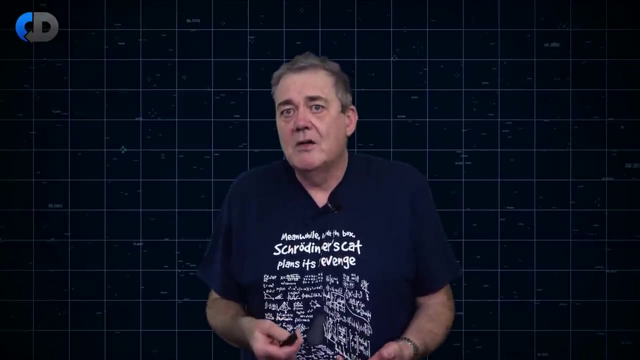 but we create these tests as little specifications of what we really want before we start, And then we use them to guide the creation of our code. If one of these tests spots a problem, we stop and correct the mistake. This is about as efficient and as high quality as we can get. 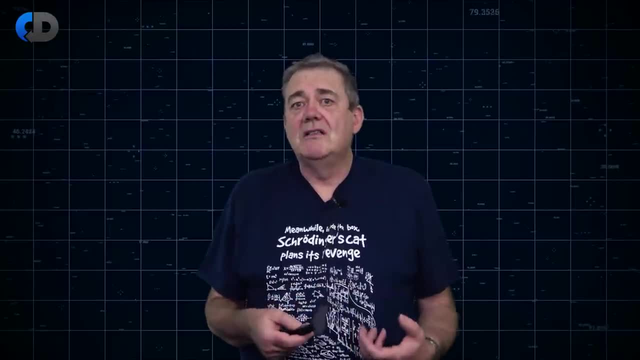 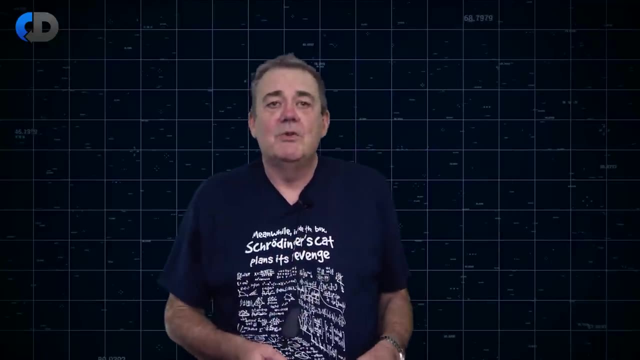 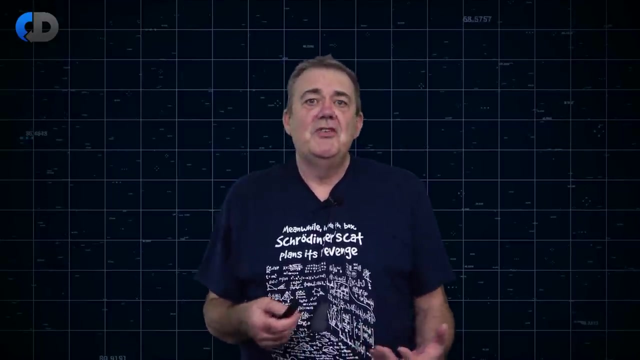 Some may think that this completely marginalises the traditional role of QA, And if you think of QA as gatekeepers staunching the flow of crap changes into production, then maybe you're right, But that is never really a good role for QA. This traditional gatekeeper approach usually ends up. in one of two bad places. depending on the priorities of the organisation, Either quality is seen as vital and then QA becomes a bottleneck slowing the pace of change. It's pretty obvious that if your QA process takes two weeks, you aren't going to be in a position to release every week. let alone every day. This has a big cost And sadly, part of that cost is a reduction in the quality of the software that we produce. You don't build high quality software by going slower. High quality comes from working in small, fast. 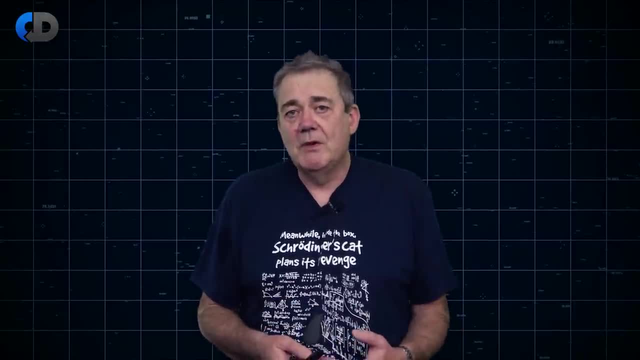 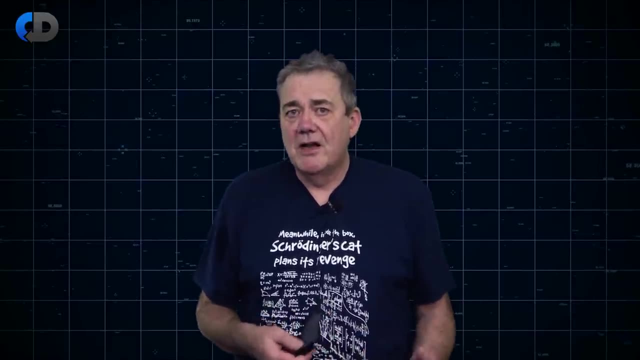 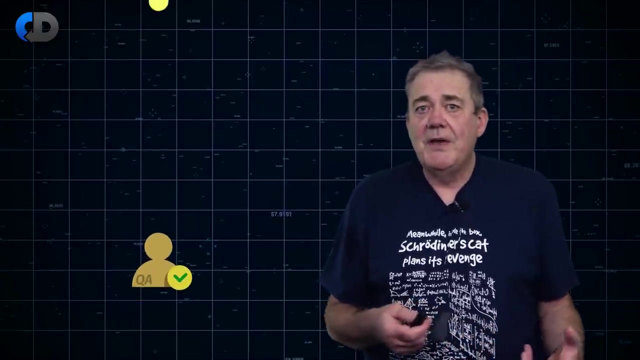 definitive steps where we can monitor the quality as we create the change. So we need to be very wary of things that slow us down. The other failure scenario is in organisations that prioritise delivery over quality. In these organisations, QA people are put into an unenviable position. They're tasked with defending quality, but they're not allowed enough time to evaluate the changes thoroughly enough. Testing time is squeezed to the point where lots of bugs slip through into production In really dysfunctional organisations. QA is then often blamed for this. Now it may sound as though I'm trying to have my cake. 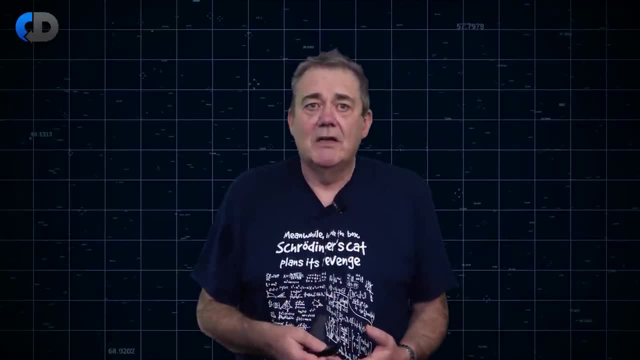 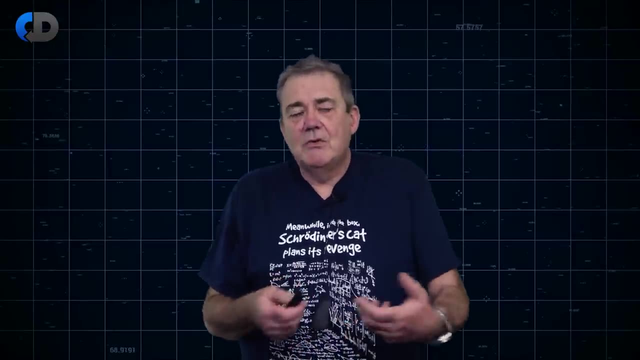 and eat it here. I said that you need to go fast to get high quality, but that going fast leads to low quality. Well, yes, that is kind of what I said. The key to unlocking this is what you mean by going fast. The trick is to spend time in the right places. Testing after the fact is the wrong place. to spend lots of time Batching up changes and then testing huge collections of change is a very low quality approach. You can't inspect quality into the system after all. 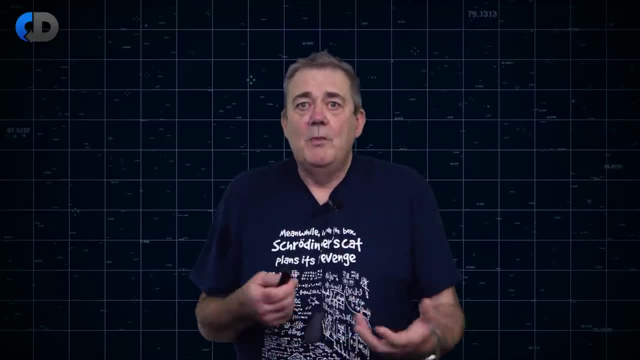 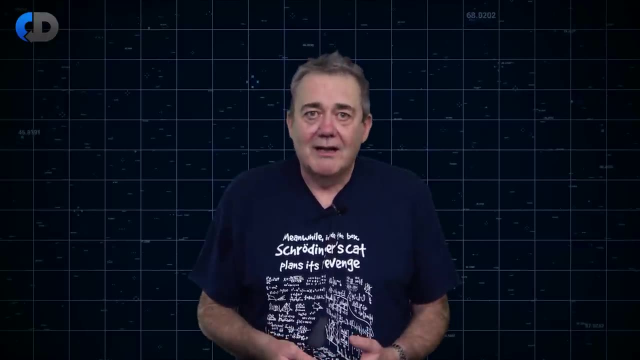 Equally not. testing and crossing your fingers, hoping that this time our genius will tell and there will be no bugs is just fantasy. Sure, you can write code like that, but it won't be any good. So we need to build quality in and we need lots of tests. 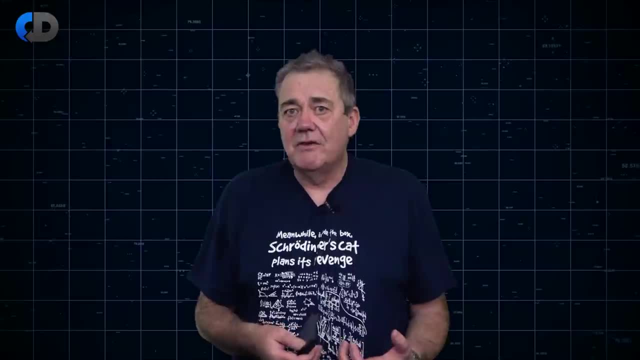 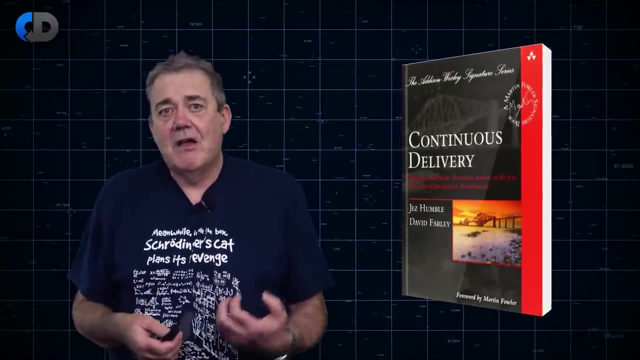 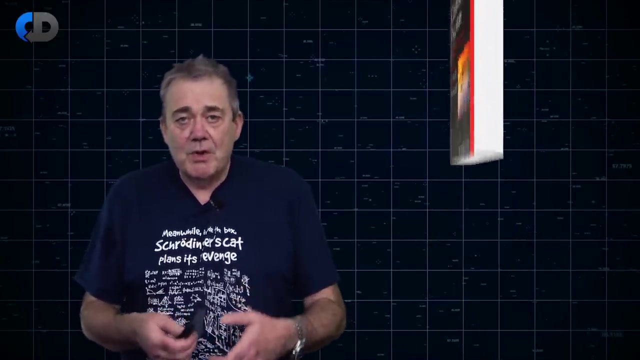 Continuous testing isn't an add-on to continuous delivery. It's a cornerstone of it. In my continuous delivery book, six out of the 15 chapters are primarily focused on different aspects of testing. Continuous delivery is aimed squarely at this problem. Our aim is not to marginalise quality. 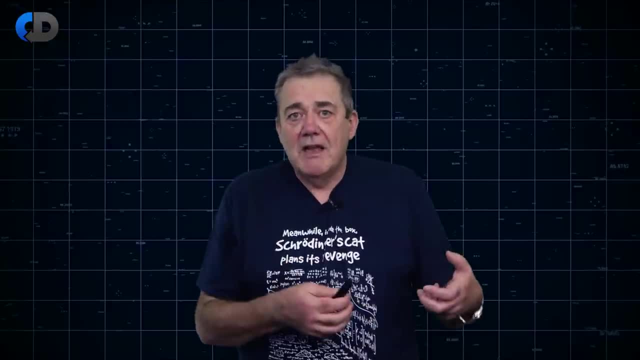 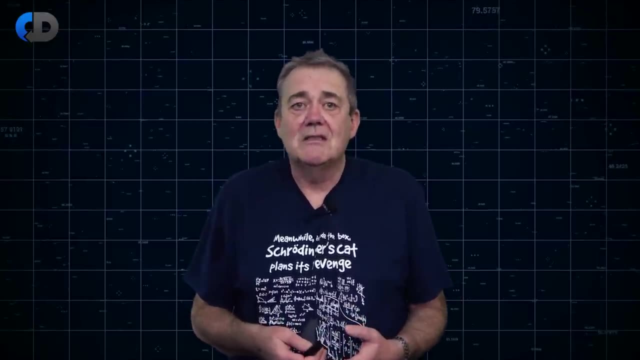 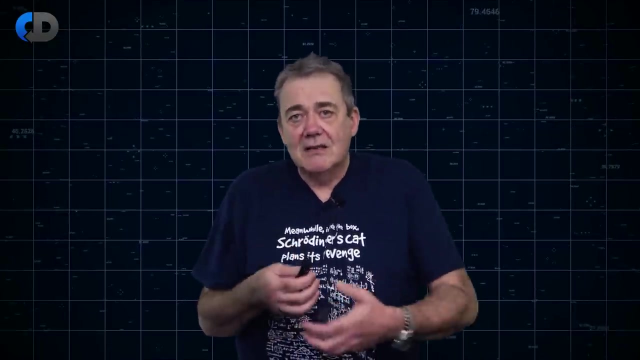 Completely the reverse. Our aim is to place quality front and centre in our development process. The whole team needs to become quality focused, maybe even quality obsessed, And this is one important role for QA professionals to take: To act as guides, experts on thinking. 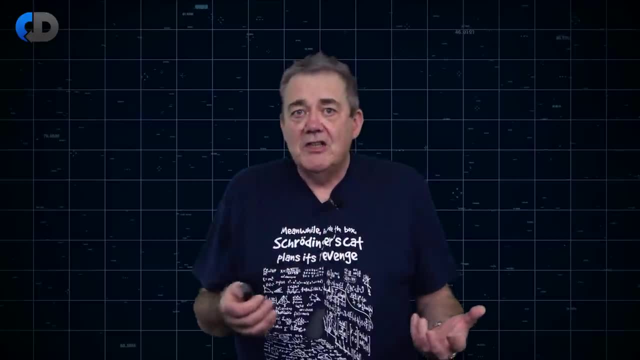 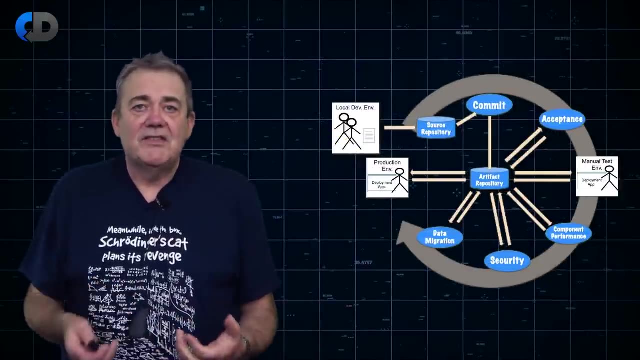 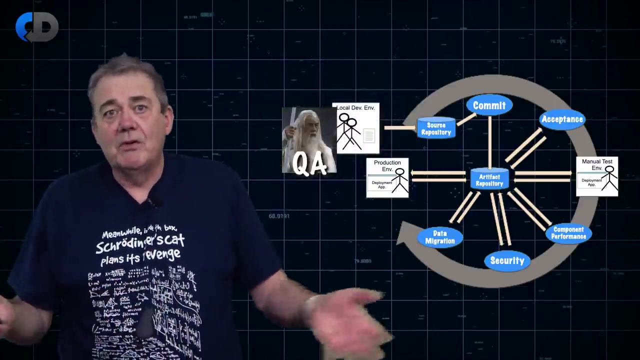 about quality and testing, Not after we've finished, but rather before we begin. This rules out a few common approaches to QA. First of all, it's a bad idea to have a separate QA team. You may have a QA community of people who share good ideas. 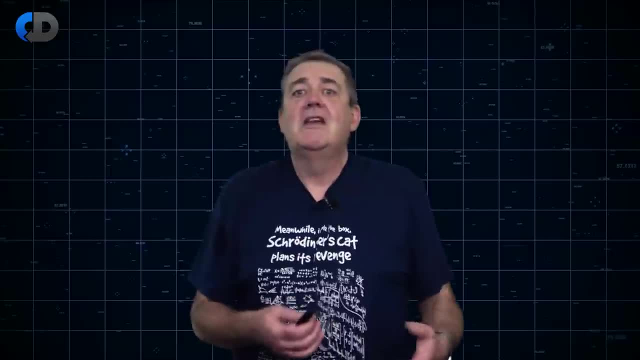 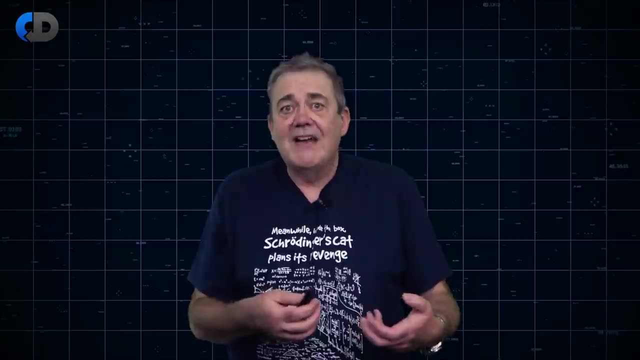 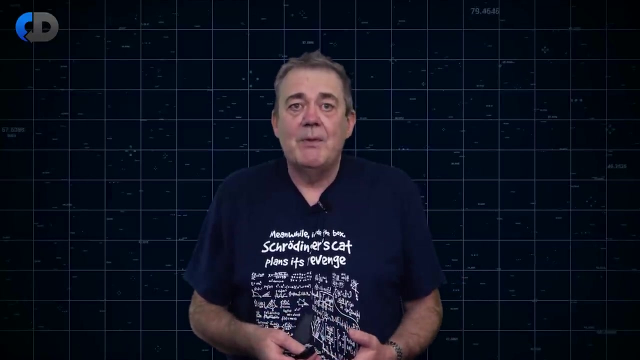 but the QA function is part of the development team. QA professionals work alongside developers, understanding new features before work on them starts and evaluating new features while they are being created, not afterwards. This way, the team can spot mistakes as they happen, rather than days, weeks or even months later. 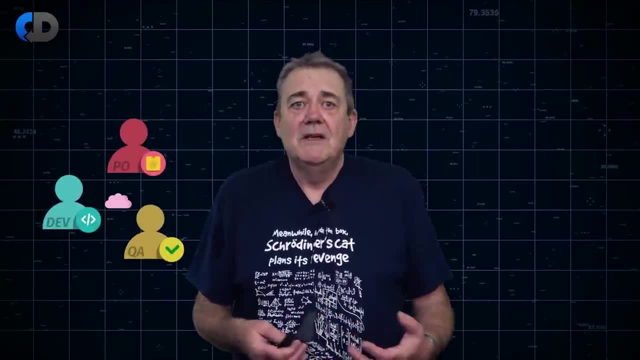 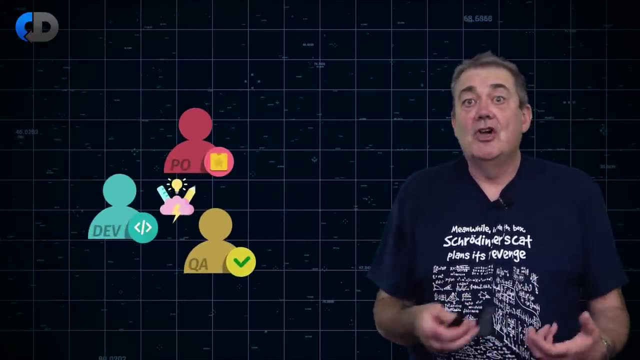 As a new feature comes in, it's a good idea to have a QA team. When it comes into the team, the team discuss it. They all work to explore and understand the new feature and what it means for users of the system. This encourages us to capture requirements. 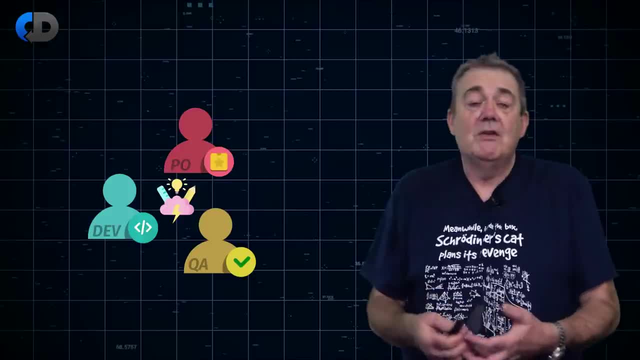 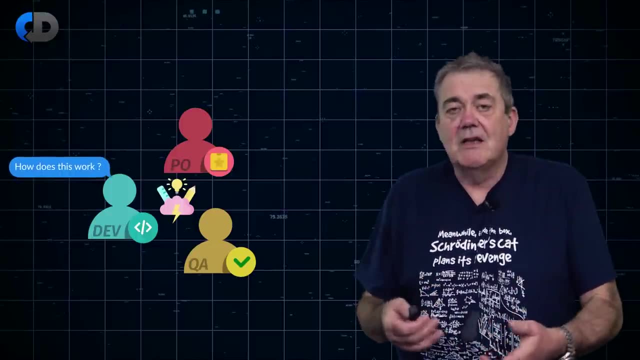 from the perspective of our users, which is a very good thing. It also means that while we're having this conversation, the developers are thinking, how does this fit into our design? And the QA folk are thinking: how do we test this? 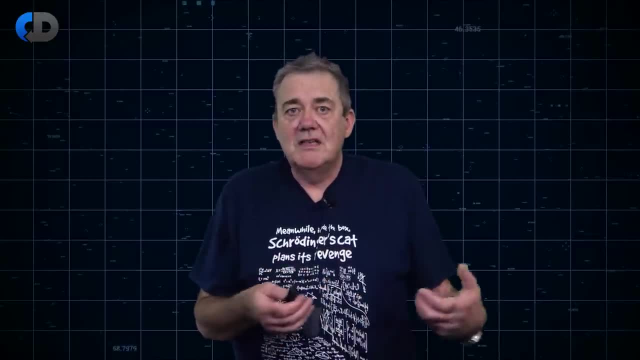 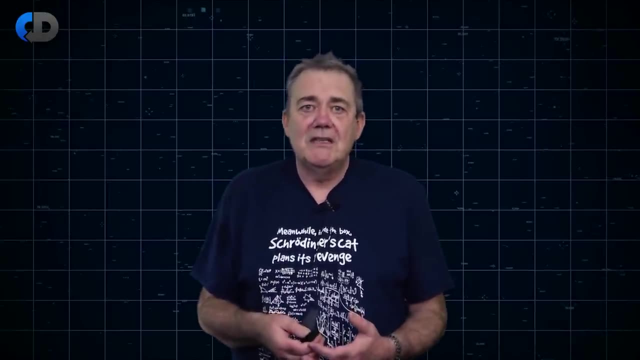 When the teams start work on the feature. my preference is that we organise a story kick-off of some kind. In BDD circles this is sometimes called the three amigos meeting. except in the teams that I worked on, there were usually four of us. 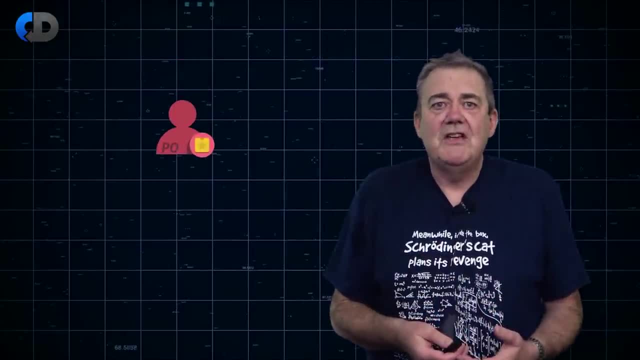 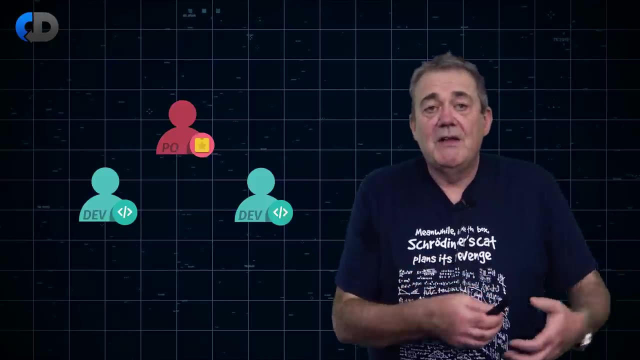 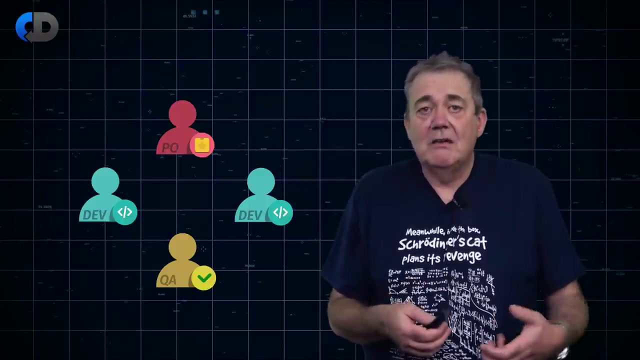 We'd have the product owner, who understands the need for the feature, the goal that we're trying to achieve with this change. We have a pair of developers who will start work on developing this new feature together, and the QA, who will act as an advisor and do any manual testing that we think is worth. 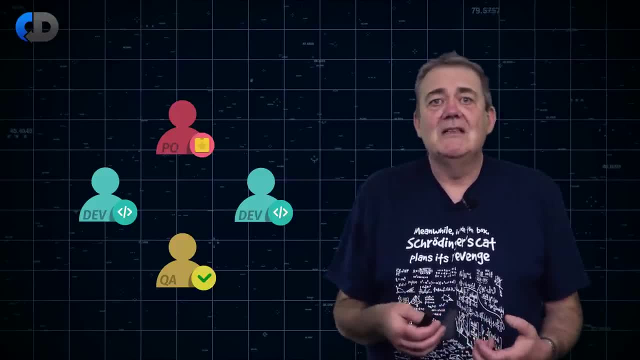 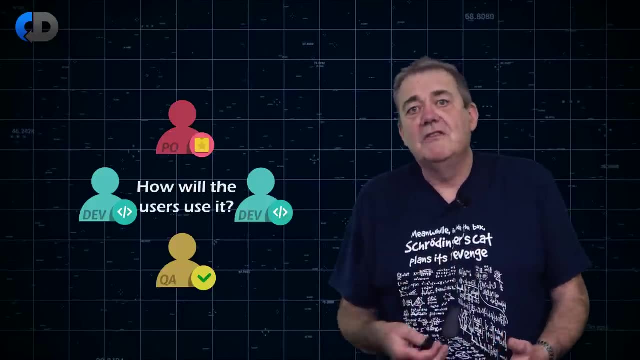 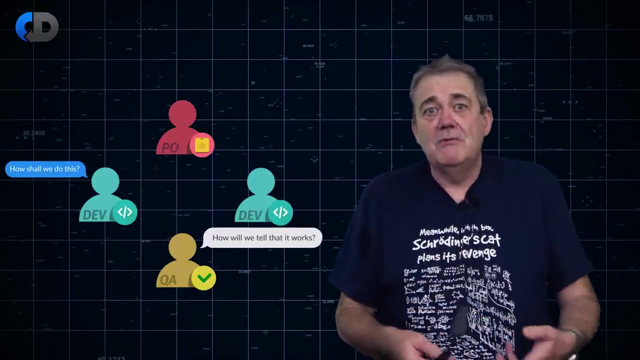 while The conversation usually begins as an exploration of the new feature, What it's for, How does this fit in with the existing system, How will the users make use of this, And so on. Then the developers and the QA start to explore how they will be able to tell that the system 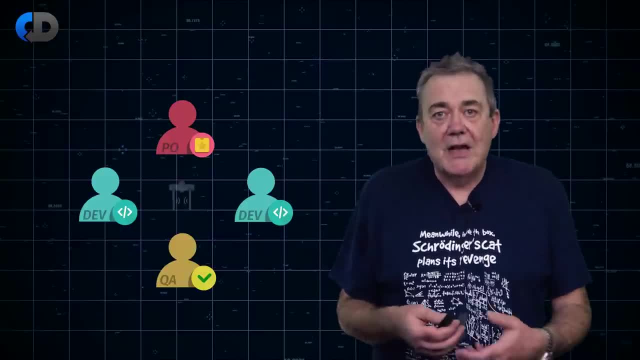 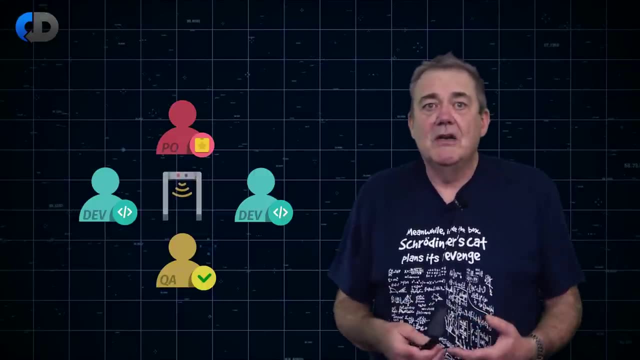 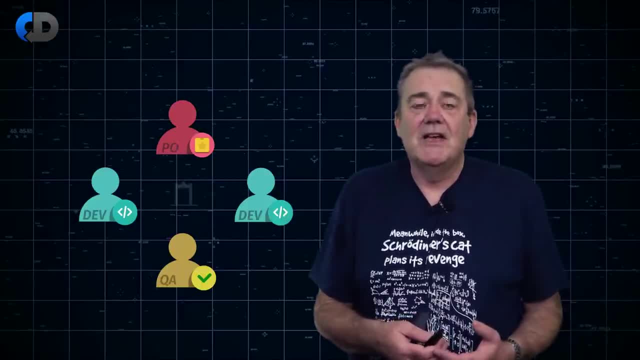 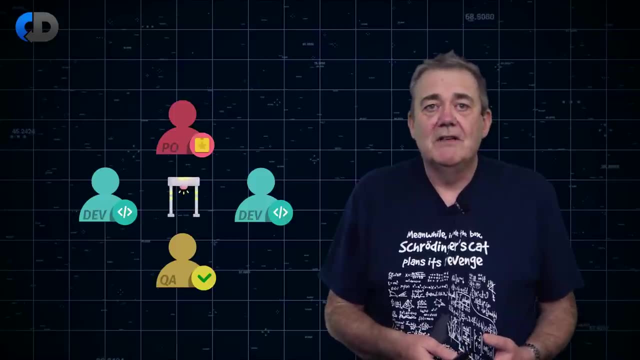 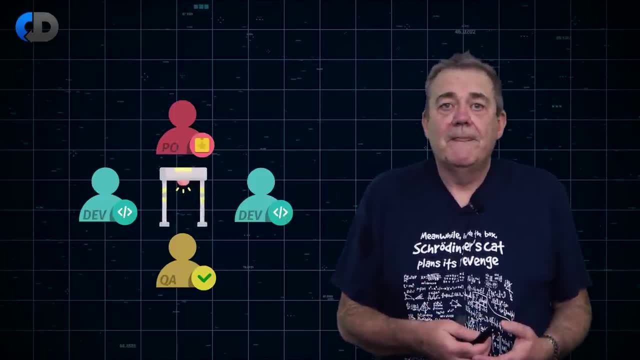 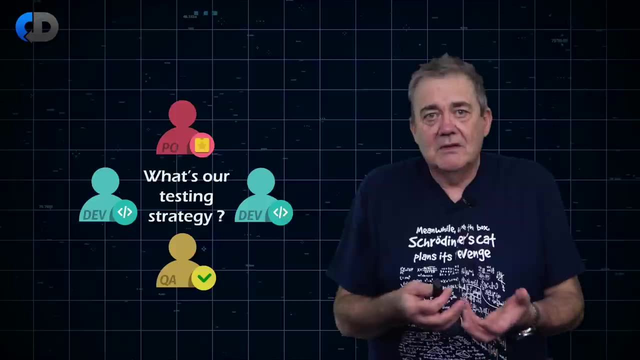 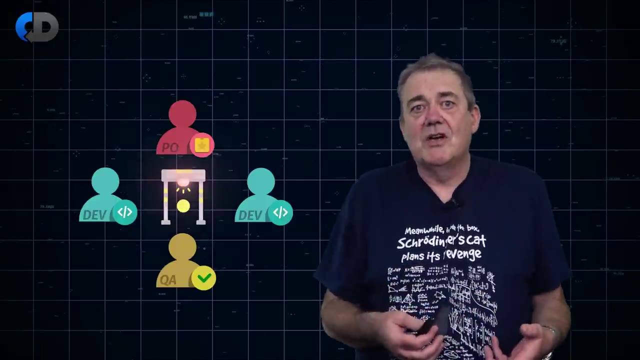 and form the acceptance criteria for the new feature. Now the developers and the QA discuss their testing strategy. They all assume that the idea is that they're going to create tests for each of these acceptance criteria, an executable specification that demonstrates and evaluates each example that they thought of. 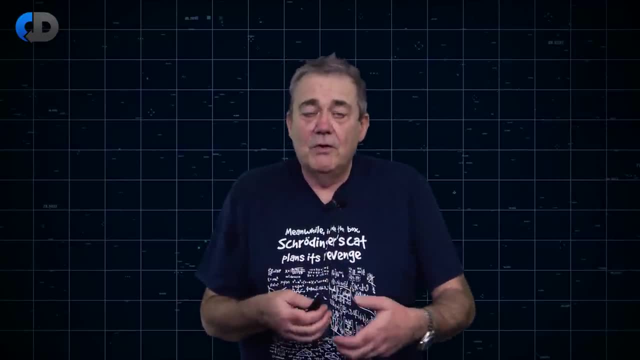 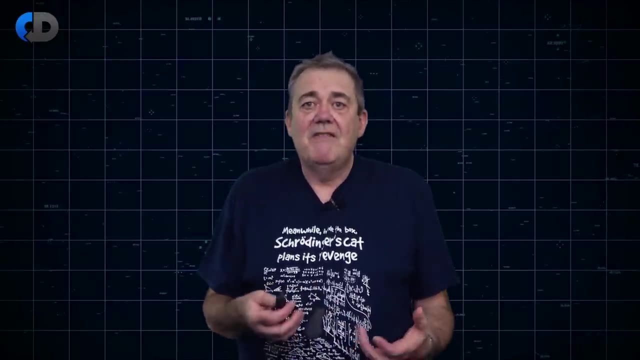 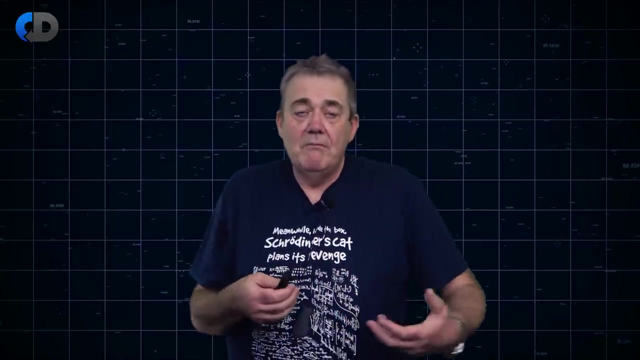 This gives them all a structured definition of done for this feature. When all of the executable specifications pass, the feature is finished. I particularly value having a QA person on the team at this point, since they often think of examples that I, as a developer, might miss. So we end up with better specifications this way. Whether the QA or the developers capture these specs as automated tests, It depends on the team and the individuals. There's nothing wrong with either approach. On the teams that I worked on, QA, people often wrote these tests. But equally, developers often wrote them too, and nearly always added to them. Even if the QA person writes the specifications, they're the developer's responsibility. After all, they are the people that will commit changes that will cause these tests to fail. 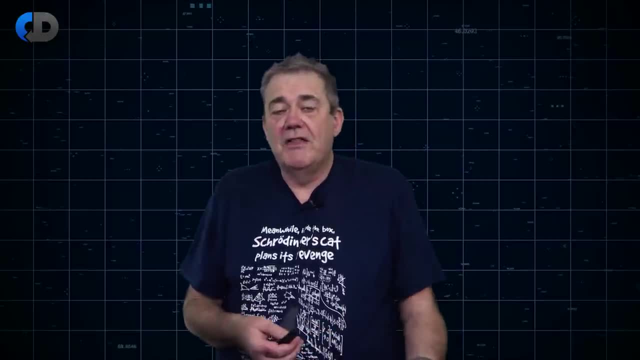 So they need to be the people who will see the result first. So they need to be the people who will see the result first. So they need to be the people who will see the result first via their deployment pipeline. This way, they can respond to failures fast. 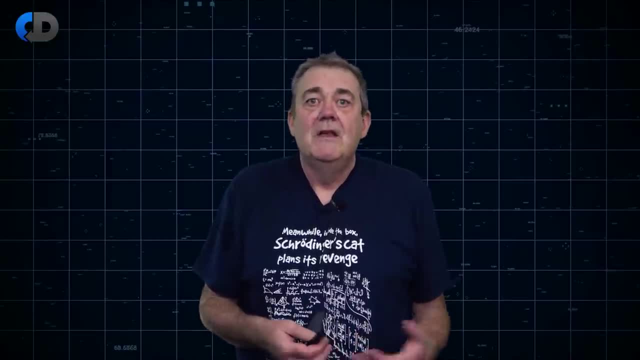 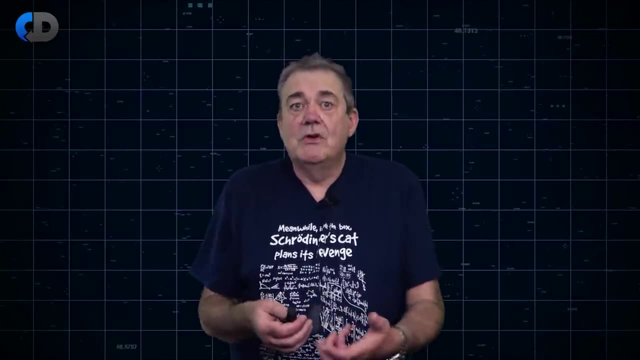 After all, why slow things down with a middleman at this point During this conversation? one of the goals is to strategize about any manual testing. It may surprise some people that I'm talking about manual testing, But I think that manual testing is really valuable in the right context. 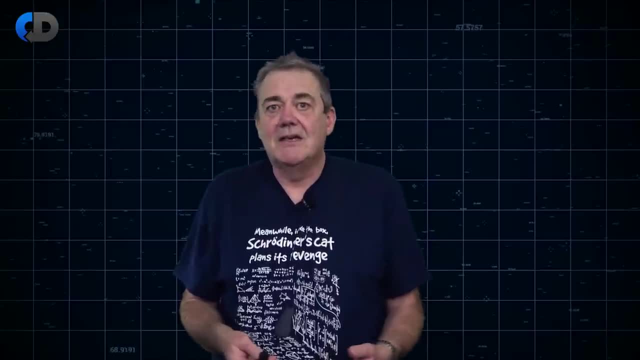 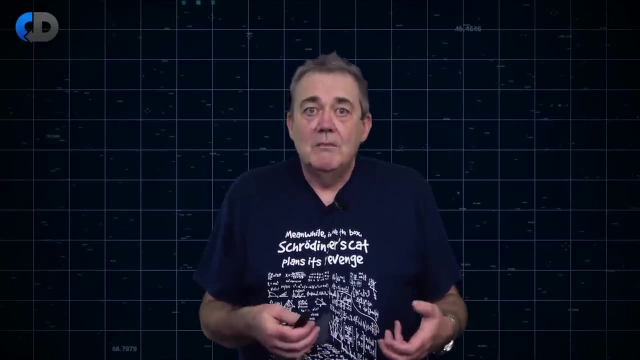 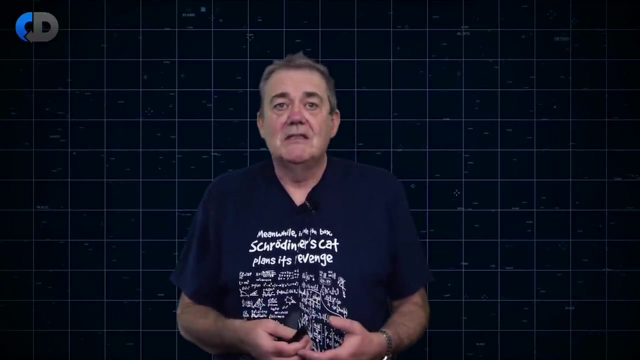 I just don't think that manual regression testing is valuable in any context. If our aim is to be efficient in delivering feedback into development teams, our goal needs to be to automate all regression testing, But there are some kinds of tests that humans are much better at. 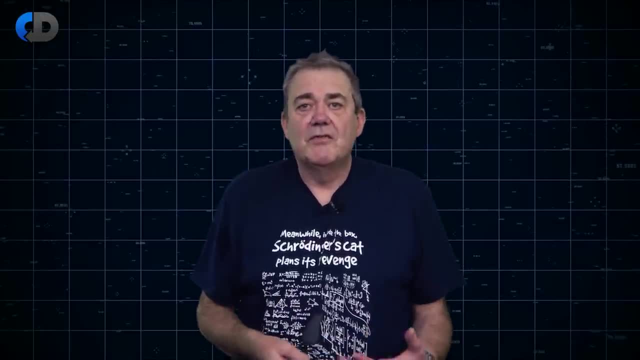 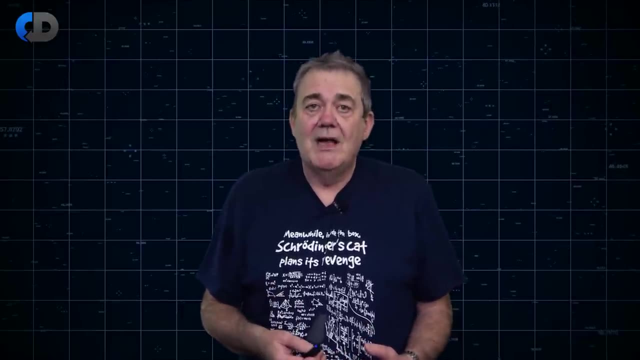 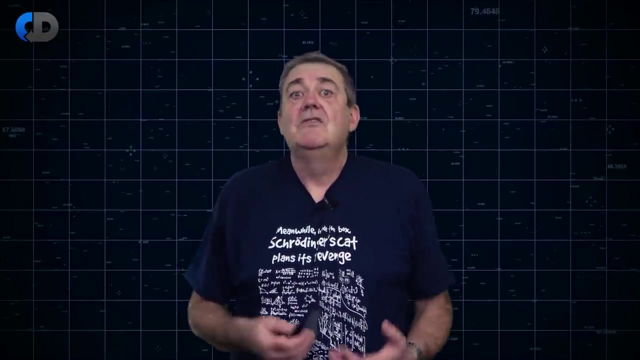 For these things, manual testing is best. If our software works, and our automated testing should assure us of that, then what humans add is: does it work well, Is it nice to use? Does it paint pictures in our minds that help us to understand what's going on? 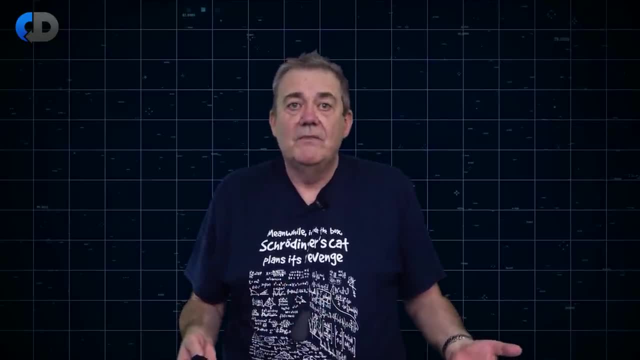 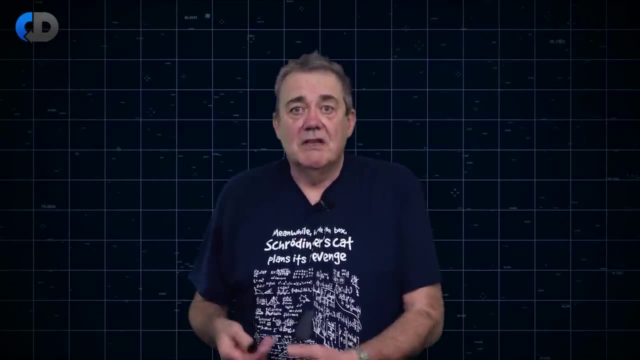 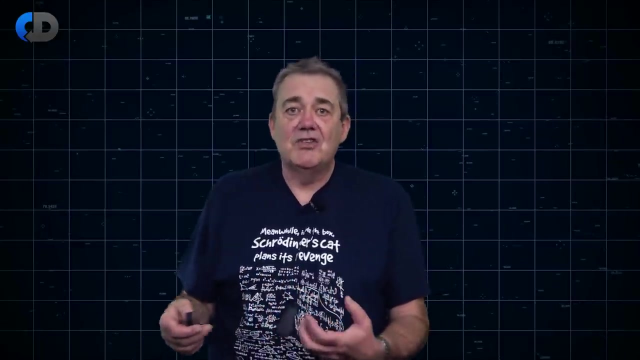 Does this new feature look good? Does it fit in with the rest of the system? This more subjective exploration of the system doesn't need to be repeated all of the time. It happens once at the time when we make the change. I think of this exploratory approach to manual testing as surfing the leading edge of change. 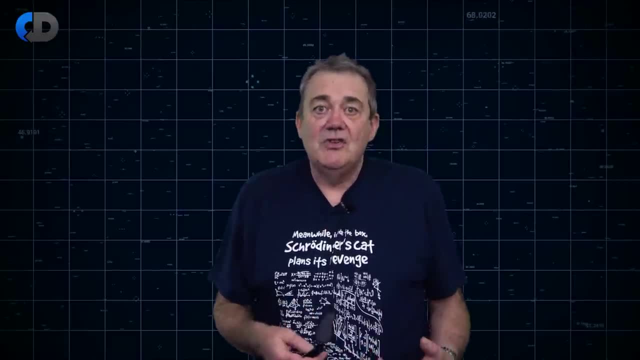 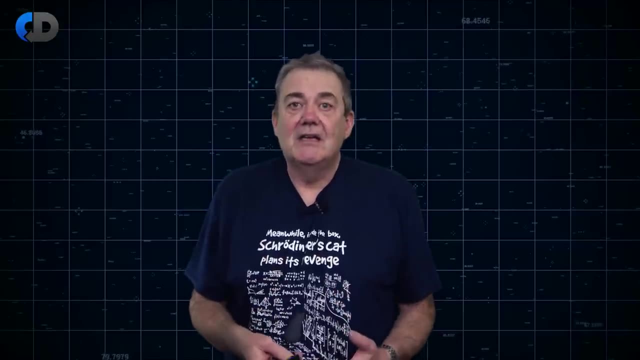 in our system, QA, people are looking at changes as they are being developed and give feedback on these changes to their dev teammates. In fact, that's part of the planning at the kickoff. Once you've done this part, I can test it. 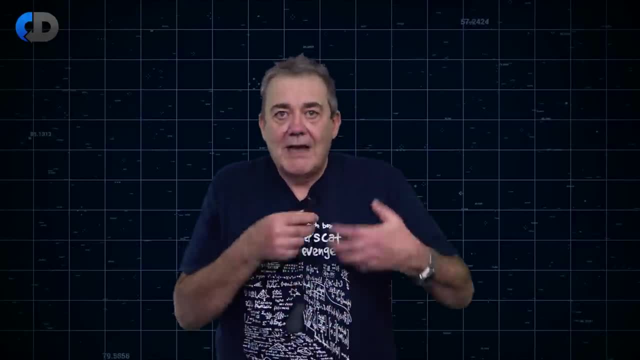 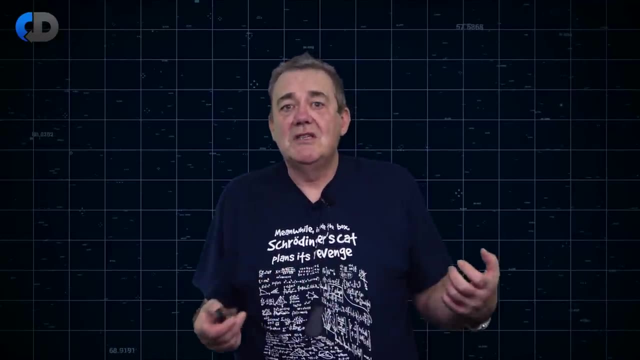 So let me know as soon as I can. Our aim is to avoid building mini-waterfalls into our development process. We don't want the developers to work on a feature until they think it's complete and then hand it over to a QA person. We want everyone to be working alongside each other on the feature as it evolves and ideally, everyone finishing at roughly the same time. So if a QA person spots a dumb mistake in the feature, they can point out the mistake to the development team while they're still working on the code. 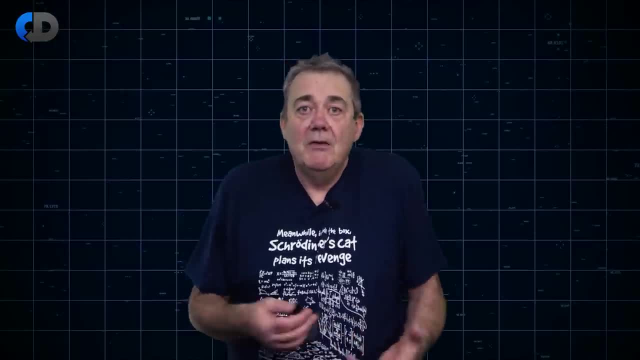 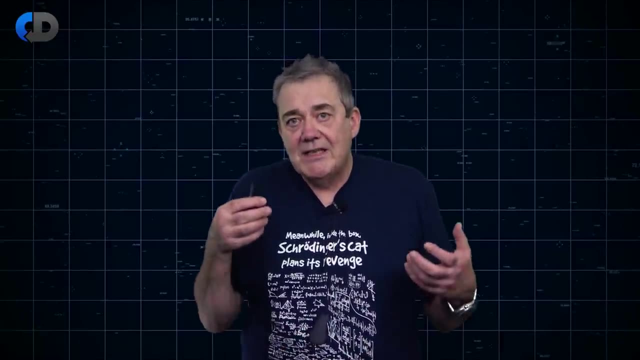 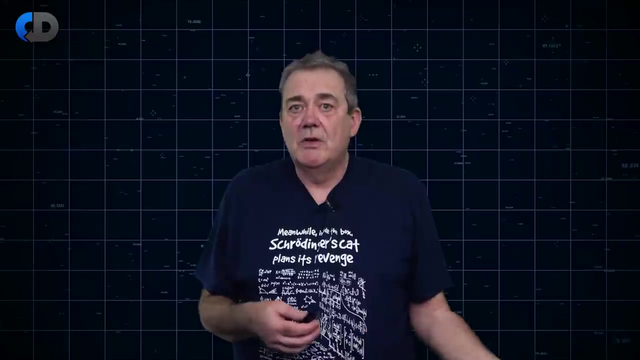 No need for a formal bug report, just have a chat. No need to wait for the feature to be finished before starting work on fixing it or on testing it. Continuous delivery is a challenging change for everyone, But it is a particularly big change for QA people, at least for those who are used to. 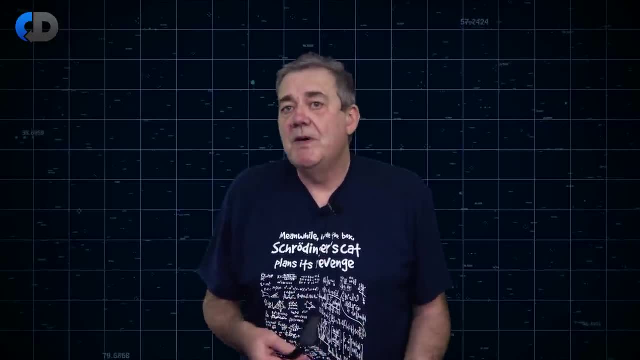 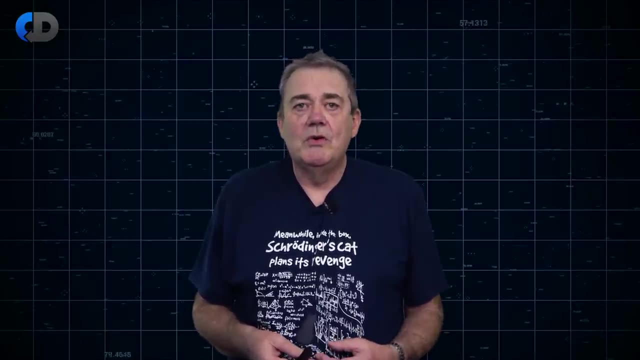 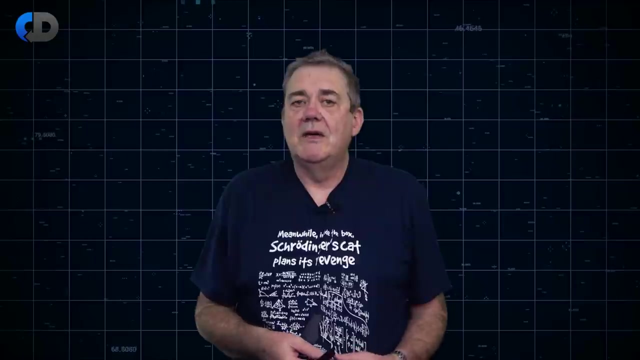 working in more traditional settings. My experience of seeing people make this transition, though, is that this is the first time I've seen it, This approach to QA is much more rewarding, and that the QA professionals that I have seen make this step would never willingly go back to the old way of doing things. 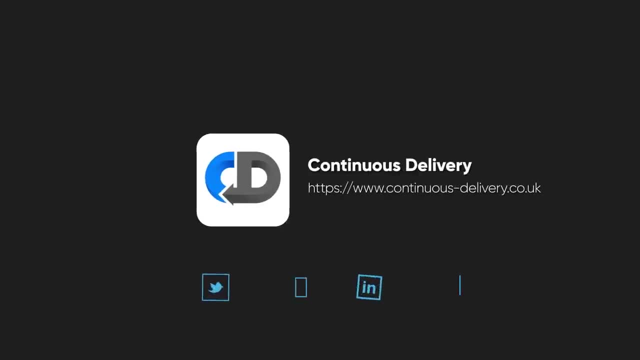 Thank you very much for your time and there are no more questions.